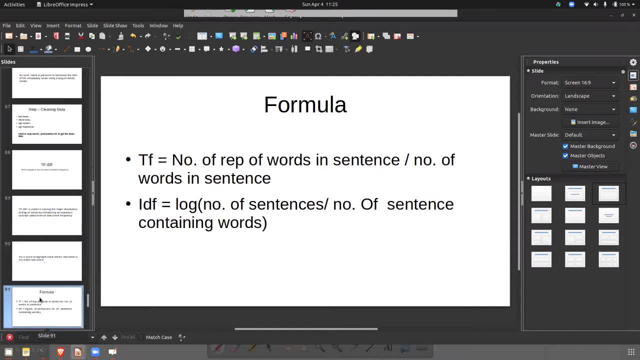 Number of repetition of word in a sentence divided by number of word in a sentence. So please note, I'm not talking about sentences, I'm talking about sentence. So sentence is nothing but one sentence at a time. So number of repetition of word in a sentence divided by number of word in a sentence. 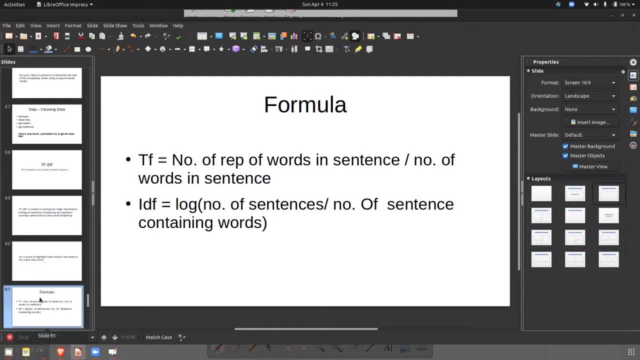 And IDF stands for number of sentences. log of Log of number of sentence divided by number of sentence containing this word. So it's okay if you don't understand. So this is the formula. Understand the formula is okay. With the help of example, I will try to make everything clear. 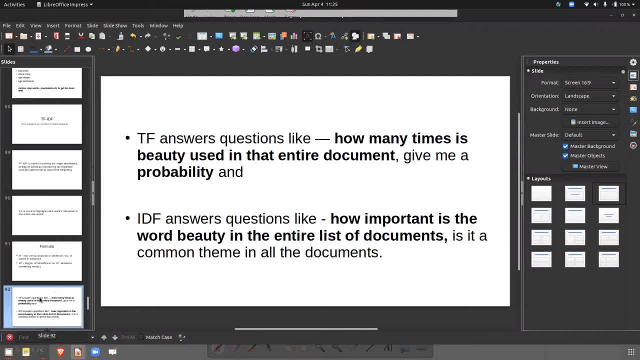 So this is the basic fundamental of TF and IDF. So TF answers questions like: how many times is the beauty used in the entire document? Suppose you have a document, So the purpose of the TF is to tell you that: how many times the beauty is used in the entire? 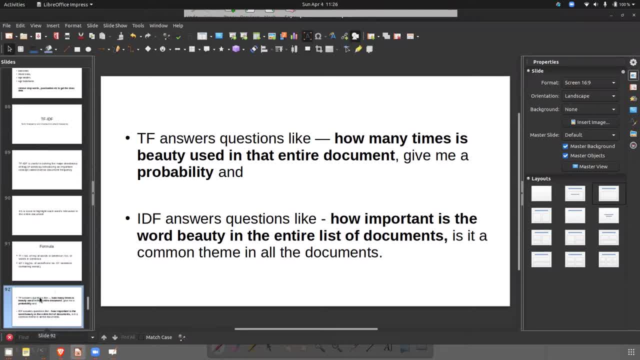 document- Give me a probability of that- Where IDF will tell you that how important is the beauty in the entire document. So the purpose of the TF is to tell you that how many times the beauty is used in the entire document. So the purpose of the TF is to tell you that how important is the word beauty in the entire. 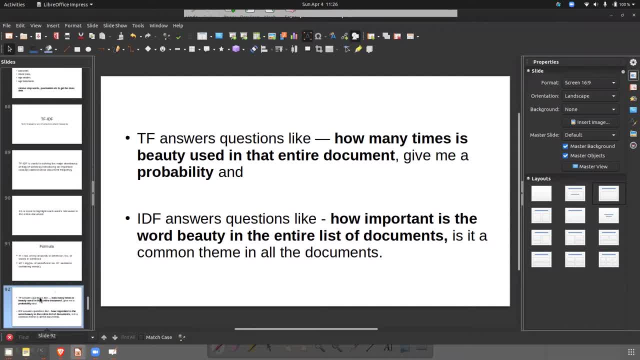 ratio document. So that is now clear. So we have TF and IDF. So TF will tell you that the word, what is the probability of that word, that is present inside a document, And IDF will give that what is the importance of that particular word in the political document. 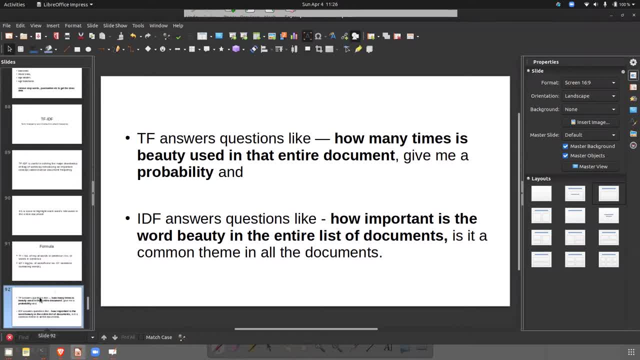 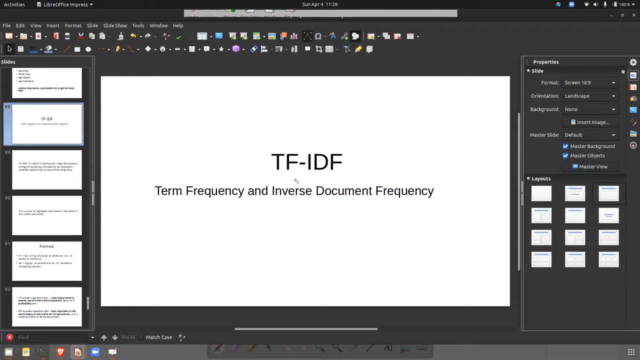 So that's why we have something called TF and IDF. So now the two terms are clear to everyone. Yes, Okay, So, Okay. so can anyone tell me that what TF is and what is IDF is? What is the main purpose of TF and IDF? 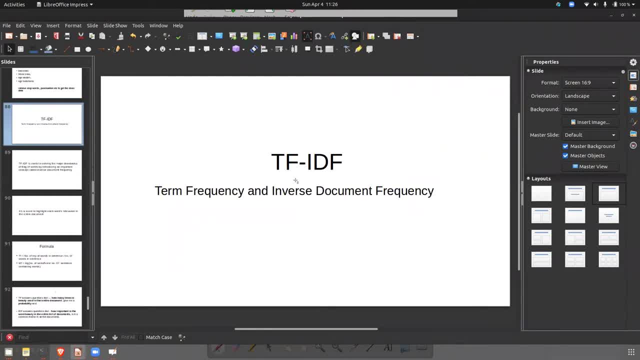 In a layman words, okay, so that everyone understand Anyone. TF is how many times that particular word is in a document, Okay, And what is IDF? How many times the word is repeated in all the documents. Okay, so TF is how many words? so suppose this is sentence that is good, for example, good. 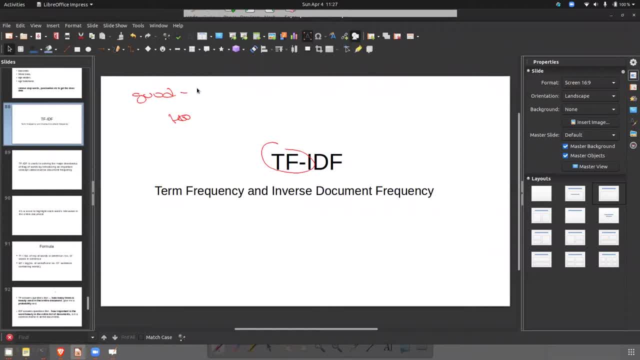 Right, So good was in the previous sentence. good was repeated in all sentences, right, So three sentences: Yes, Boy was in one sentence and girl was in one sentence, For example. okay, Now TF will tell you that how many times is good is present. 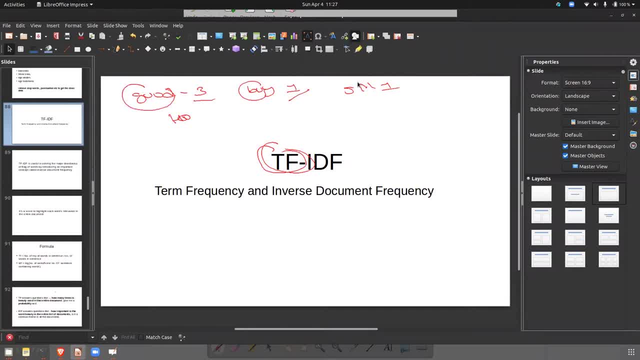 So good, is present basically three times: Boy was present for one time and then girl was present for one time. So this is nothing but TF. So this is clear to everyone. TF is clear to everyone. TF is for each document. Yeah, it was for a single document. 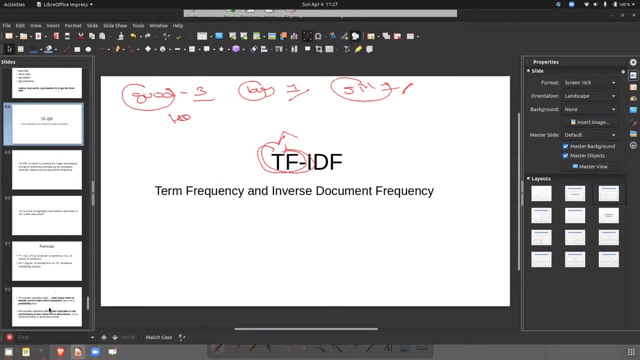 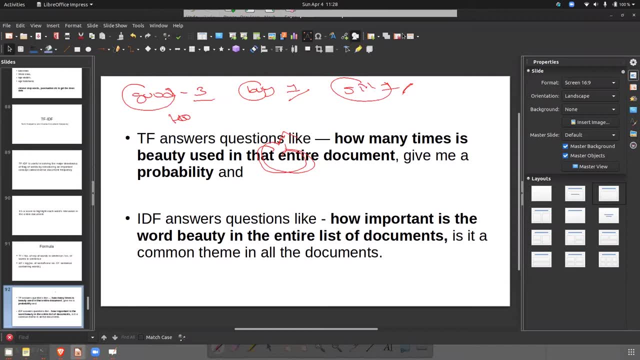 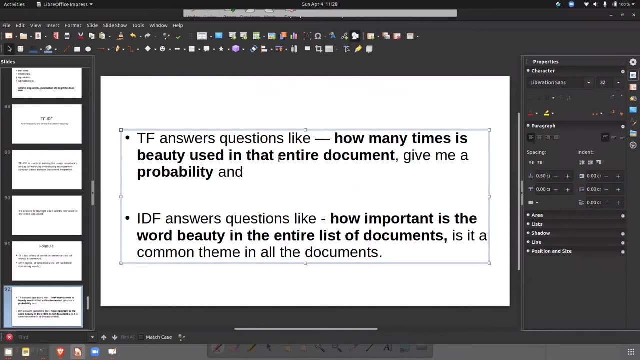 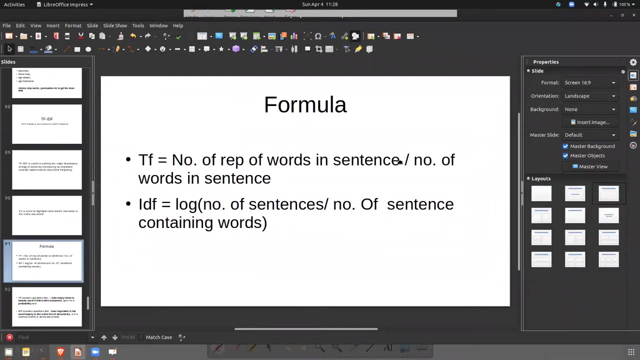 So term frequency in: no, not for the. so okay, let's, let's, let's try to See. See this: how many times a beauty used in the entire document. Okay, so, okay, let's try to see the formula. So: number of repetitions of one sentence in the number of repetitions of number of words in a sentence. 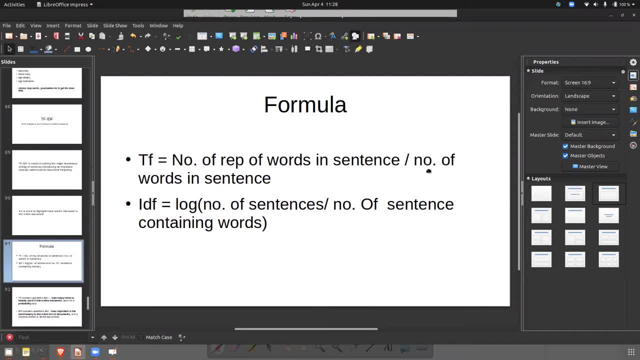 Okay, number of repetitions of words in a sentence. Yeah, so basically, it's for basically each document. Yes, correct, It's for each document. So basically, good boy and girl. So good is present, Exactly Good is present in that. 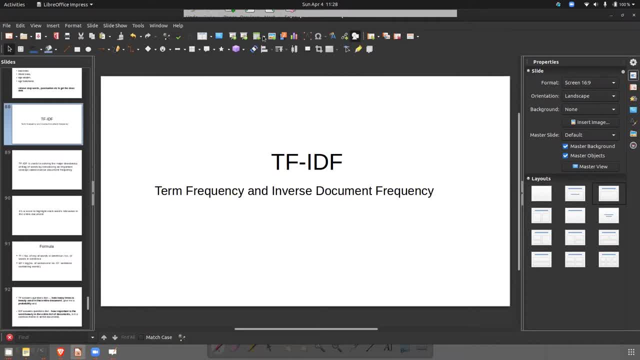 So in that document goes with one time, Good was present for one time, Boy was present for one time and girl was present for zero time. So TF, IDF will tell you that how the probability of that word in a particular sentence, TF, is clear to everyone. 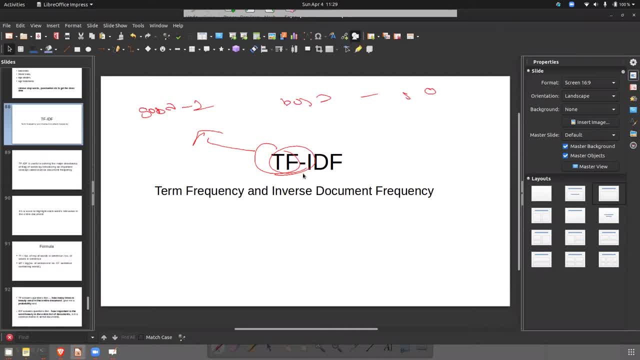 Yes, So if I've confused you. So basically, TF will calculate that That particular, What is the probability of that word in that particular sentence? That's it Okay. so what is the probability of what in that particular sentence? This is what you mean by TF. 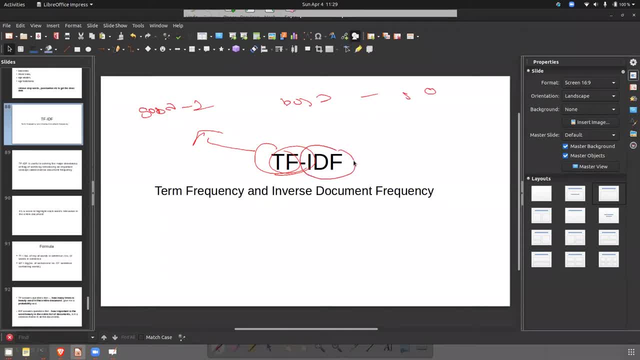 No idea. The job of the idea is to tell that Which word is important. Which word is important. Okay, whether good is important, boy is important or girl is important. That is a job for idea. Now it's clear. TF will give the frequency. 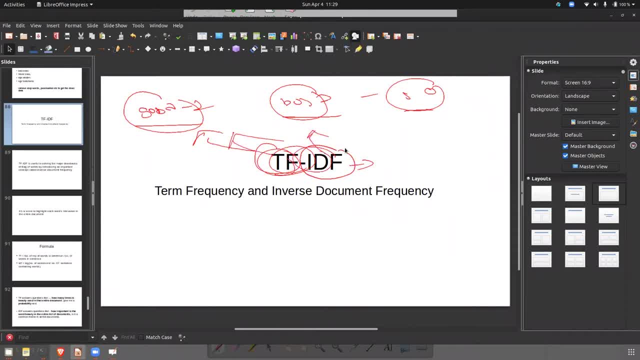 Idea will give you that which word is more important than which word. Simple definition. Now it's clear to everyone. Yeah, Yeah, Okay, Let's try to see the example, Then I think it will be more clear. Okay, So everyone is wondering how it is happening. 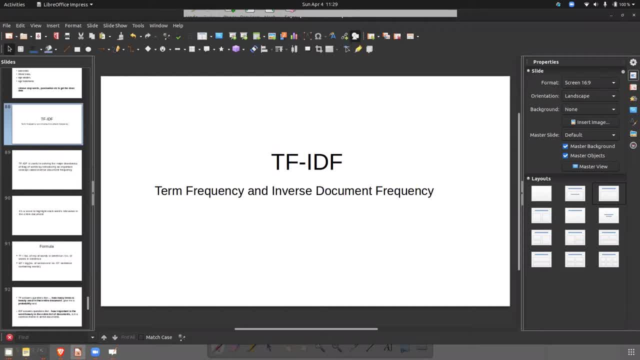 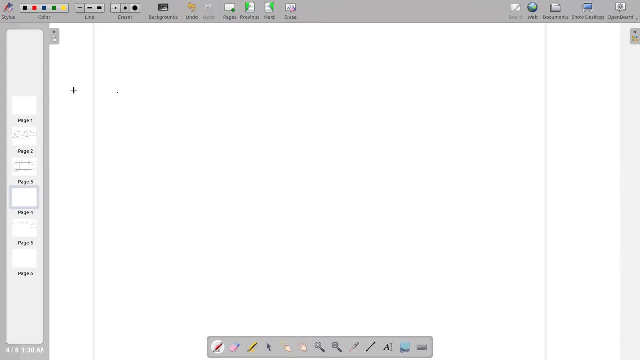 So let's try to see with the help of an example. Okay, So let's talk about TF IDF. So I think everybody remember the sentence or the first example that we took, So sentence one, So TF IDF. So first let's see the formula. 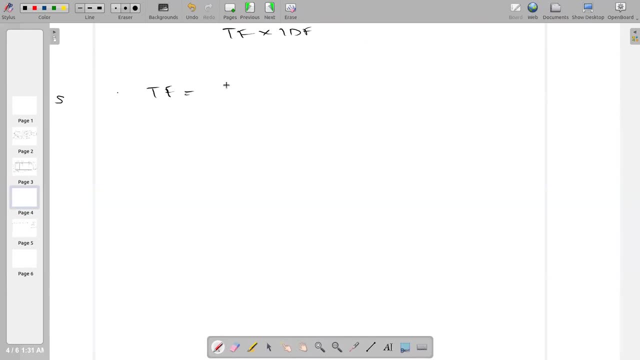 Okay. So TF stands for number of repetition of words in sentence, So in a sentence Divided by number of word in a sentence. So number of word in a sentence And the formula for TF, IDF is log of. Okay, So remember this is log of number of sentences. 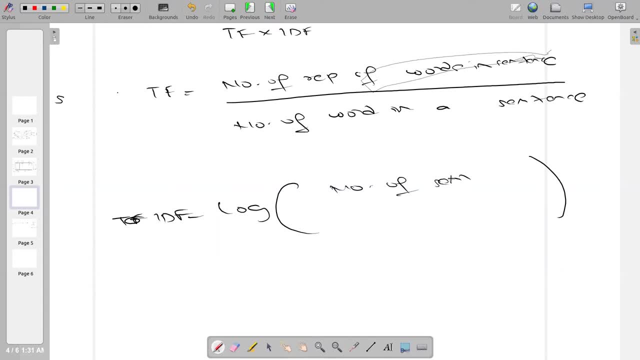 So, basically, how many sentences we have? number of sentences divided by number of sentences containing word. Number of sentence sentences containing the word Containing the word. Okay, So let's try to see this. So let's go to the new page and let let's try to convert. 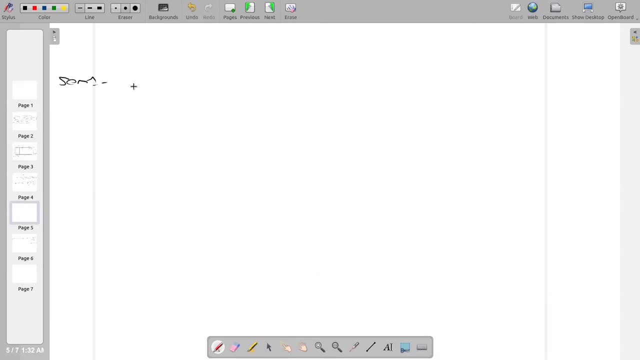 So the sentence one was Good boy, So I am thinking boy, so i am taking after cleaning, okay, so sentence two was good, good girl, and sentence three was boy girl and good. so first what we have to do is we have to calculate a tf. 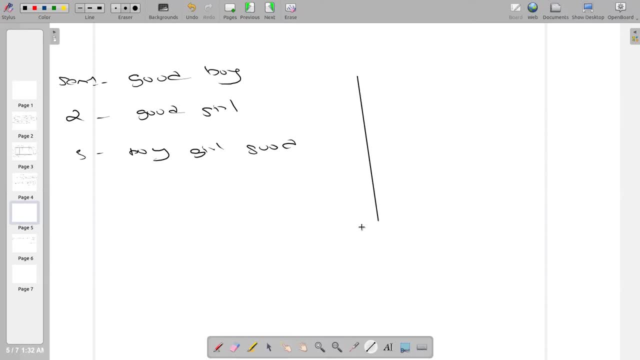 so we have to calculate. let's try to calculate a tf now. so basically, this is a thing we have, okay. so here also, you have to create a vocabulary, okay. so the first step, what you have to do, is you have to create a vocabulary. so can anyone tell me what will be present in the vocabulary? 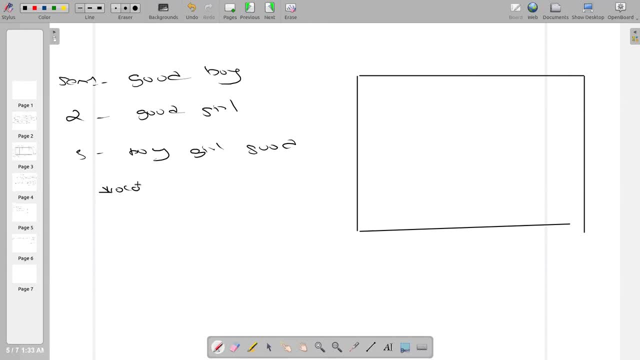 which are words really present in vocabulary: good boy and girl, good boy and girl. so basically, what we have to do is now this: features only we have to consider for tf also, for idf also, because these are the features that we are looking for. so let's try to draw a few lines. 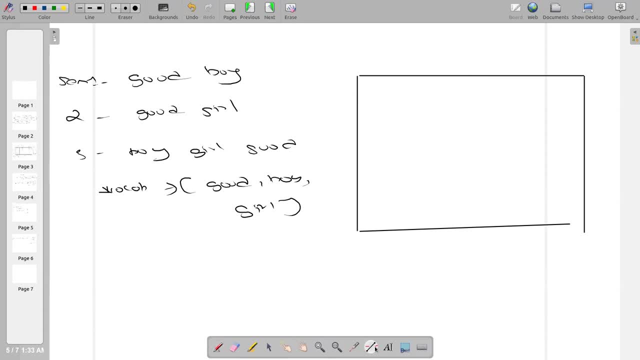 so this is basically for the words, this is for the sentence one, sentence two and sentence three, and we just partition this, okay, and then? so sentence one, two and three, we have the words called as good boy and girl. so let's go with the definition. okay, so we are calculating tf now. so the definition. 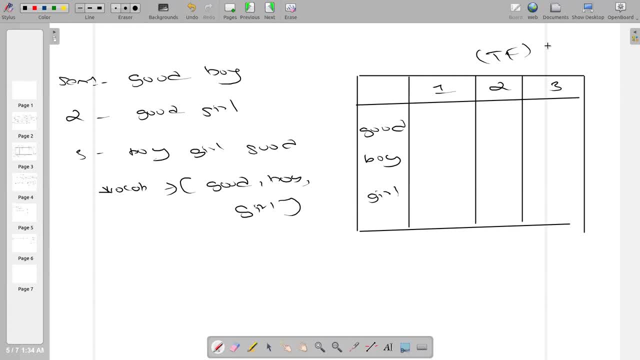 for tf is number of repetition of words in a sentence. so let's go to sentence one, so good is repeated how many times sentence one? one, one and how many. so the divided by a number of words in a sentence. so what is the number of word in a sentence two? so the answer is one by two. for this, 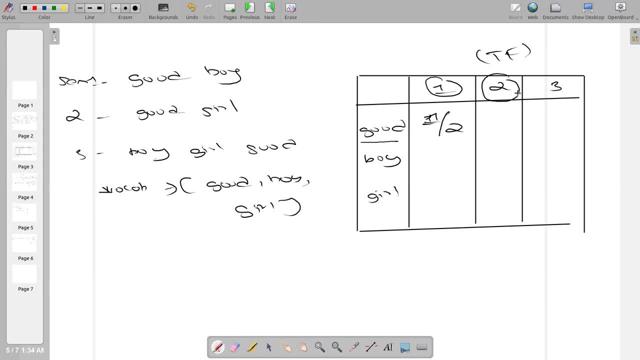 particular thing. let's go to the second sentence one by two. yeah, exactly one by two. let's go to the third sentence, one by three, one by three. let's go to the boy now. one by two, one by two, zero, zero. one by three, one by three, then then zero, zero. 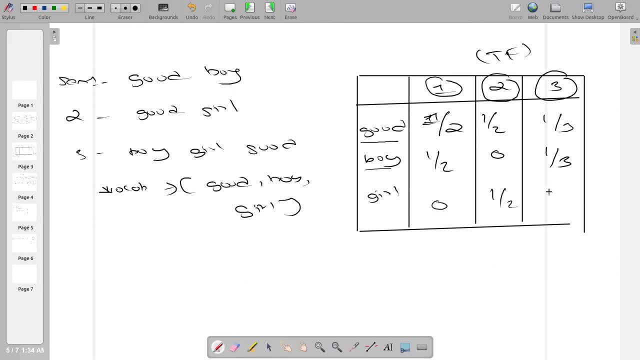 one by two, one by two, one by three, one by three. this is nothing but tf. so for each word you are calculating the term frequency. that's it. so this tf is clear to everyone. so this is called as tf table, you can see. so, for all the features, the term frequency. 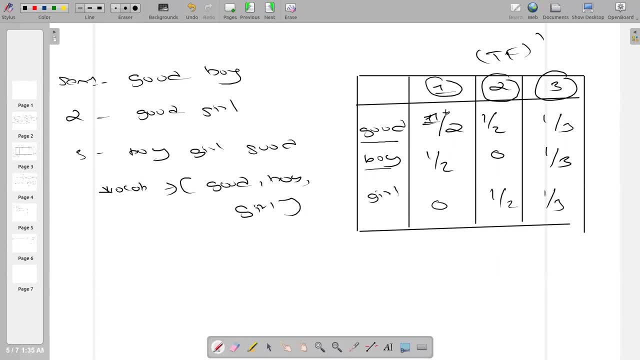 has been calculated for good in sentence one: what is the term frequency one by two for good? sentence two: what is the term frequency one by two and stuff like this. so this is clear to everyone. tf is clear to everyone. yeah, okay, now let's go to idf. what do you mean by idf? so let me try to create one more box here. 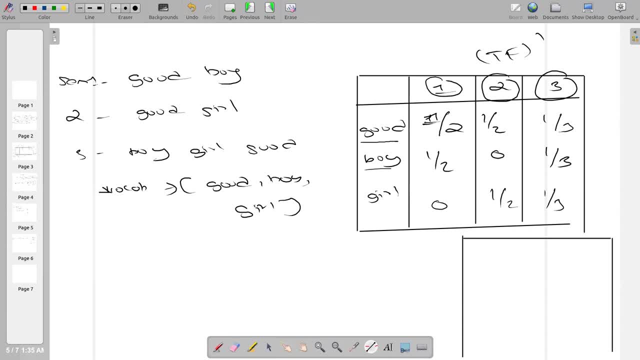 so basically, idf is for the words. okay, so idf is for the words, okay. so, uh, how many features are there? that is good boy. good, let's try to create tf for each word now. so idf for each word. no, idf for each word now. okay, so the formula for idf is log off, so i'll put log here. 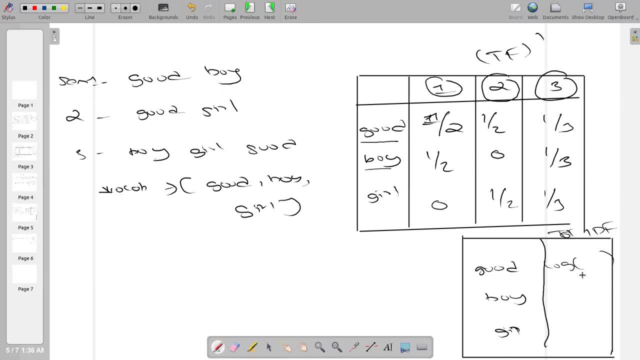 in a bracket. number of sentences, so how divided by number of sentences containing words: three. so good is present in how many sentences one, two, three. so this will become three. what is log of one? zero, zero? okay, so log of one is zero. let's go to boy now. number of sentences: three. how many times sentence present about the boy? 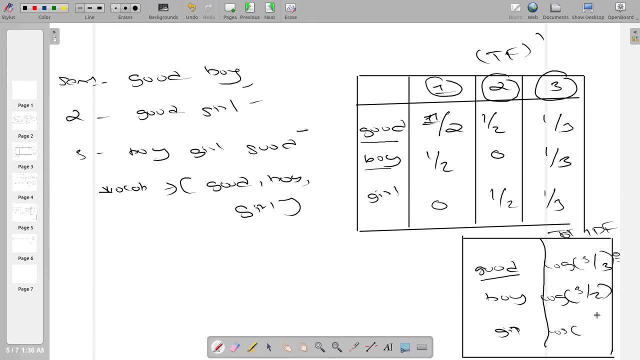 two, how, what? what about the girl? um, three by two, three, three by two. okay, so this is tf, this is idf. so, basically, what is happening for good? what is the value? value, zero, zero. for boy. what is the value? say some value, okay, some value, some positive. 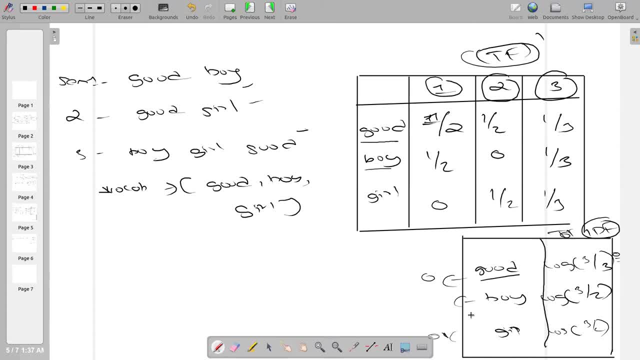 value and this is some value. so the weightage is given to which one? now, boy, boy and girl, the weightage of good is eliminated directly. this is the importance of tf, idf. now, with the algorithm, with the algorithm, it figured out that this good is present in all the sentences. 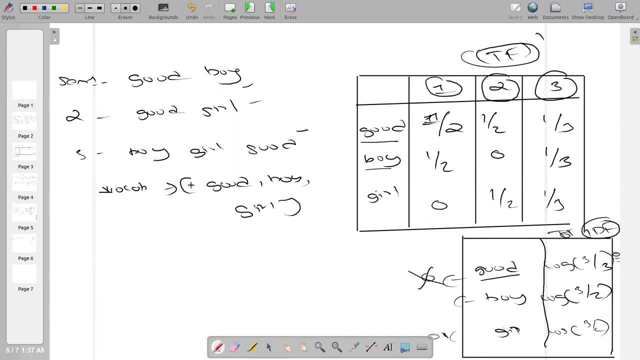 so, basically, this will not give me, this will not help me to give any, uh any output. so basically, make good as zero and give the weightage to boy and girl. okay, so how? how? this will be converted into a proper tabular form. so this is the formula. so let me draw a proper, proper. 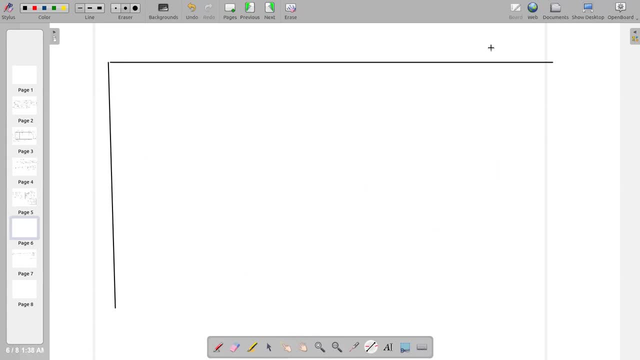 data for you and how many features are there? if i'm not on, there were three features. okay, so feature one, feature two and feature three, so let's go to switch one. so basically, this is a good, this is boy and this is girl. sentence one: you have tf. 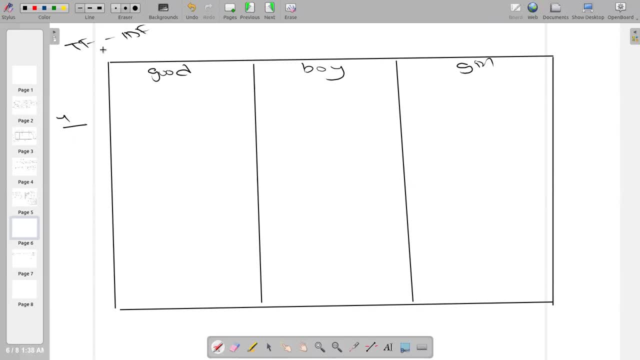 idea. so tf, idf in a tabular form will look something like tf into idf. okay, what i mean to say is: so what was the term frequency for good in sentence one? one by two, one by two, one by two into what is the idea for good? zero, zero. what about? 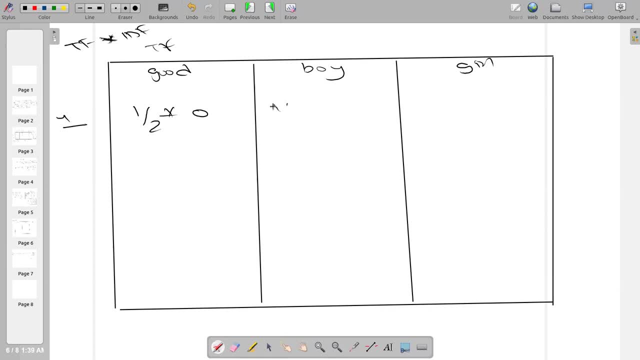 boy one by two into log of three by two. one by two into what is the idea for good, zero, zero. what about boy one by two into log of three by two. one by two into log of three by two for the girl? i think zero, yes, yeah, because, because the tf for the girl was zero in the first sentence. 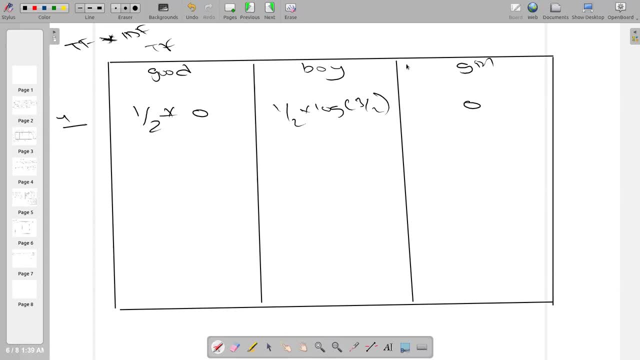 right, yeah, so it is zero. so let's go to sentence two. good, was again one by two into, into zero. boy was zero, if i'm not wrong. yeah, and the girl was one by two into log of three by two. and for sentence three, this is again one by two into zero, basically one by three into. 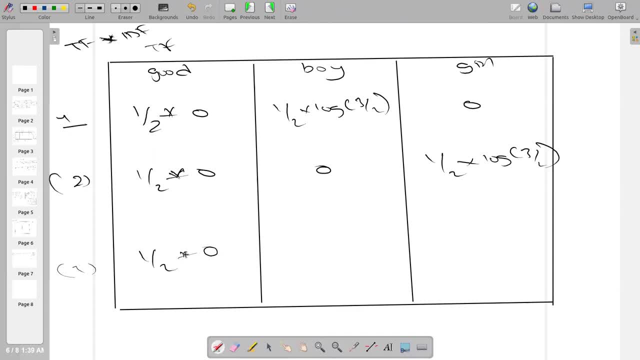 zero. okay, boys, what? one by two into log three by two, one by three into three by two, one by three, and this is also one by three into log three by two. yeah, so, basically, if you convert this, this board will is converted to zero. now, right, yes or no? 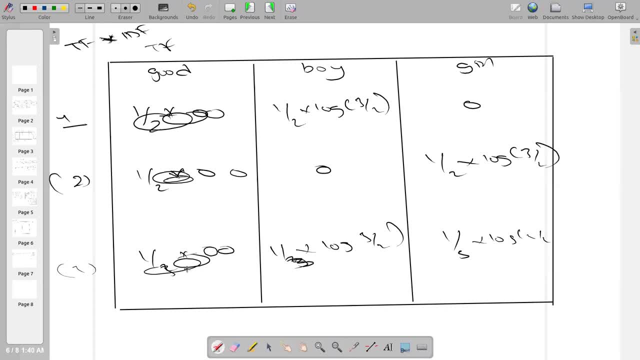 So to which two features the more importance given now both and good and good is not given any importance now. So this is the importance of using TF IDF. Now it's clear to everyone that What is it? You can see, Yes, I. 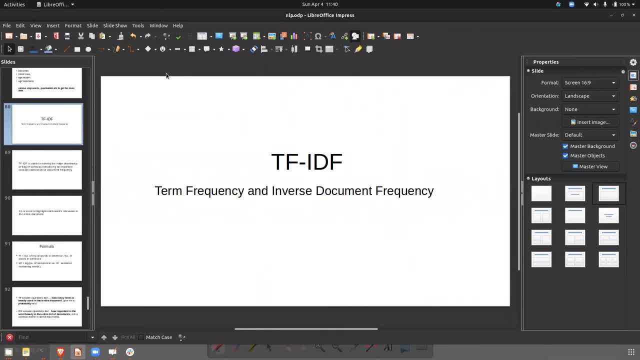 after the: and can you just look and draw, So sorry, After doing this tf IDF, like, can we look at the tables and treated and drop it by 11.. Okay, Leona, I said So. I'd say that TF there 11. And then in those cases where grows viewer. 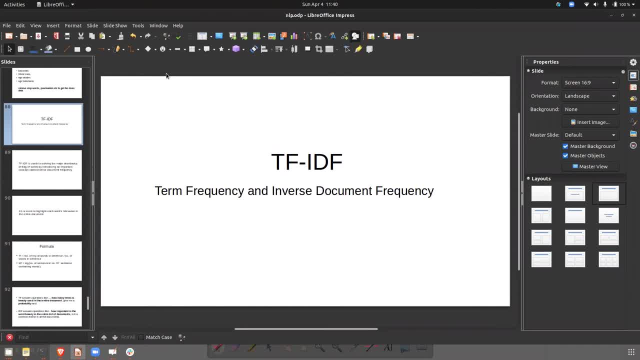 That identity deleterious. just they see it in order. So again there, hyoid and to сем üç Was telling me as well: here, So your chart, here that non beliefs. So it's very clear what 11 columns, ah, okay, okay, you're saying, okay, it is up to you whether you want to drop or not, it's up. 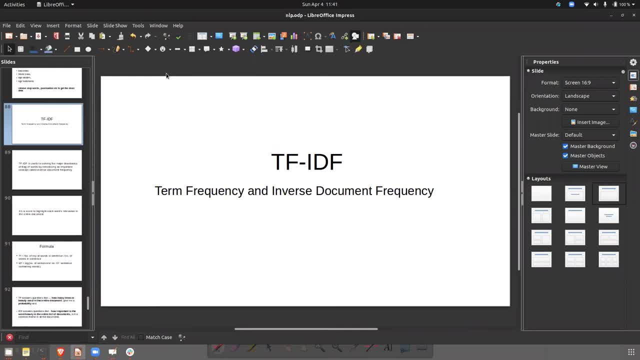 to you but basically, basically: uh, we never drop the columns, okay, so what you can do is: yes, but the problem is that we have taken only three sentences, okay, so don't not for these sentences. good is coming, zero, zero, zero. but what if you have a number of? you have ten thousand sentences. 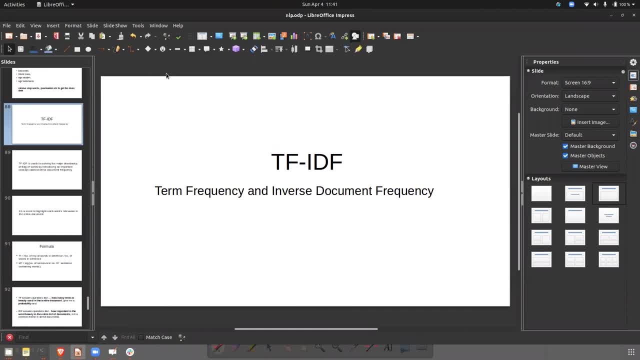 that case will never happen, right? yeah, for this particular example, good was present, all the sentences, so that's why it was coming zero, zero, zero. so that's why you can tell that, okay, sentence one is so good, word is not relevant. but try to understand that in a real world you will have. 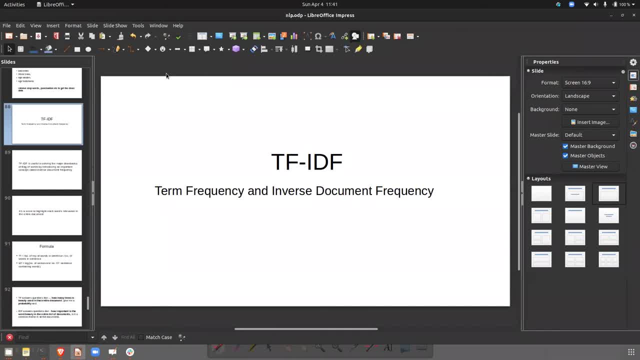 you will not have three rows if you have ten thousand rows and in that all the rows will be not zeros. getting my point? yeah, there, we will have some. so basically, basically, uh, the weightage of good will decrease the good, the weightage of good will be there, but 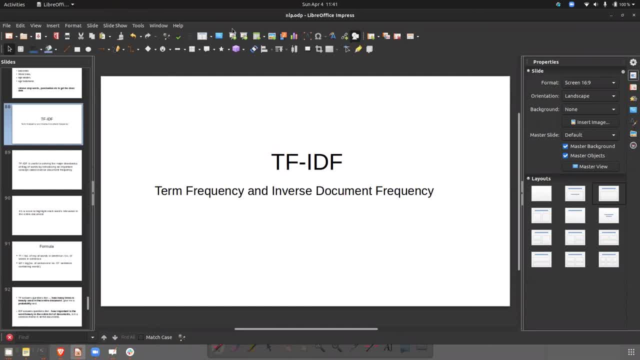 it will decrease. for example: uh, the weightage of good will be zero point, the weightage of the example will be zero point, and it okay. the weightage of the good will be 0.2. the weightage of boy will be 0.8. so from this my machine learning will understand: okay, give a small. 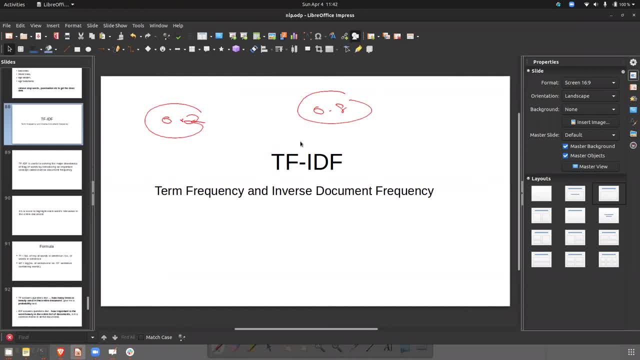 weightage to good, but a large weightage to 0.8, so this will happen in the real case scenario. getting my point? yeah, so yes, the dropping of the column is not not a good idea. i hope. i hope you have cleared the answer. yes, yes, so we will try to see with the help of an example and it will be more clear, okay. 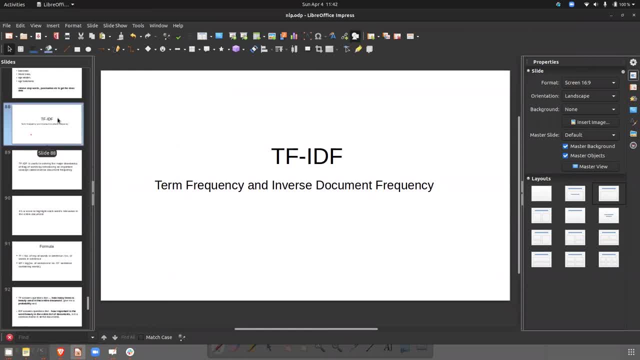 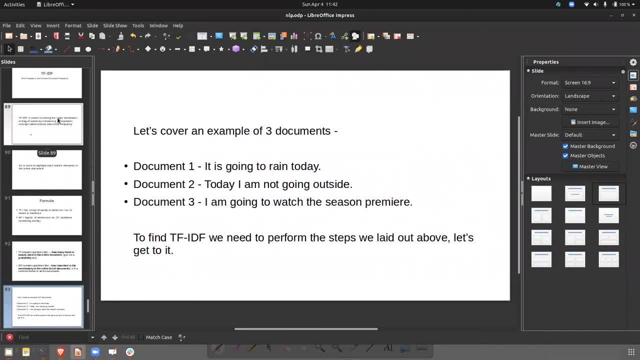 so yes, okay, okay, so, uh, let's cover an example of three documents. okay, so i've taken a different document now to get a better understanding, so that we can understand much better. so basically, i have document one and it is going to rain today. document two: today i am not going outside. and documentaries: i am going to watch the season. 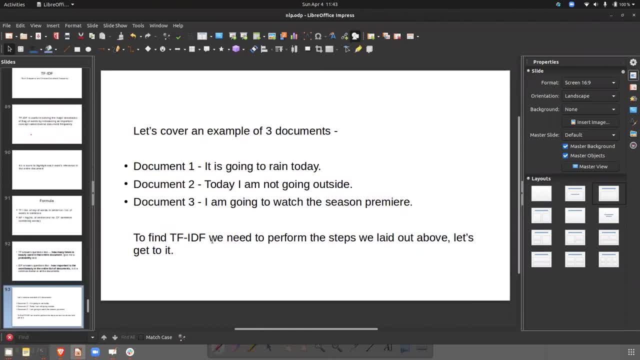 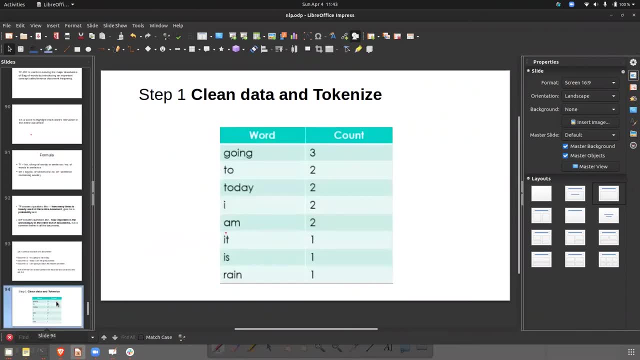 premiere. so to find tf, idf, we need to perform step. we laid out our let's go get to it, okay. so let's go to the step. so this is what we are getting. so we are cleaning the text and we are just doing a word count. that's it, okay. we are just cleaning up, cleaning up data and we are. 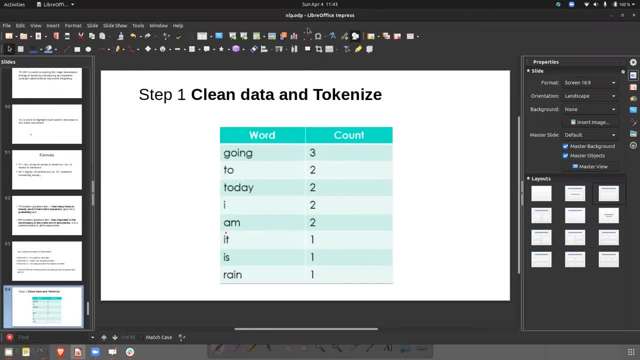 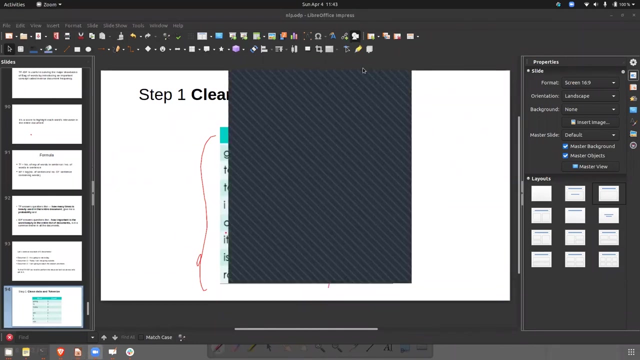 doing the word count. so this is what. can anyone tell me? this is what. this is not tf. this is not tf. okay, this is not tf. just tell me about this and then this is nothing but vocabulary. this is not what this is. this is vocabulary. okay, okay. 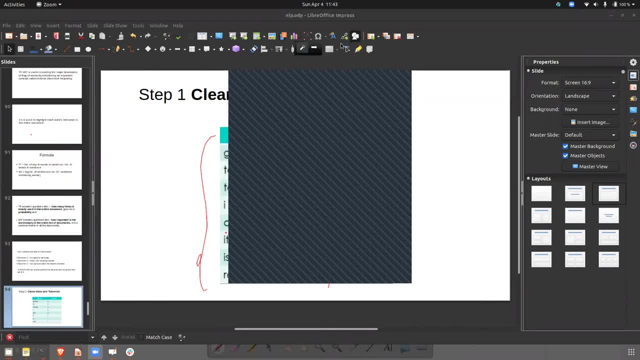 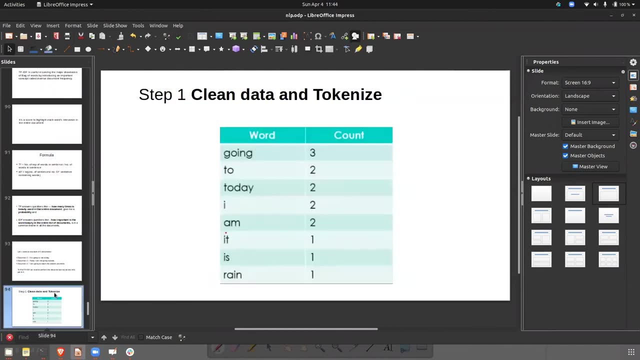 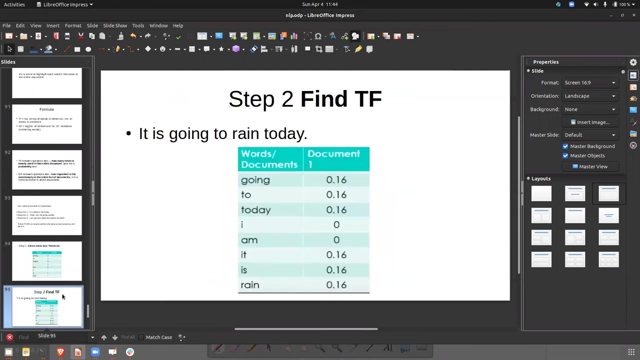 let me also clarify first: okay, so let's see, going to today i am, it's rain, okay, let's move this. so basically, okay, this is nothing but a sentence, or what organization you can say and how i tell everybody is repeating it, something like that. so this is not vocabulary yet. okay, so this is step two. so basically, 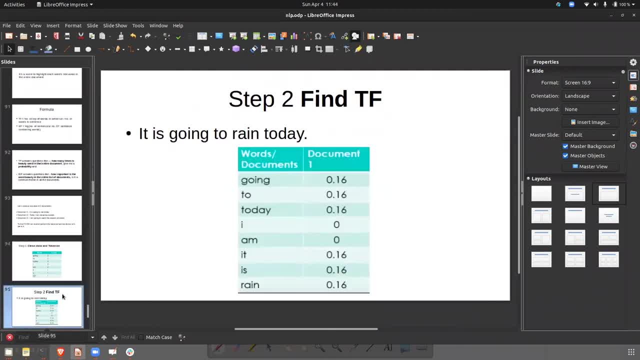 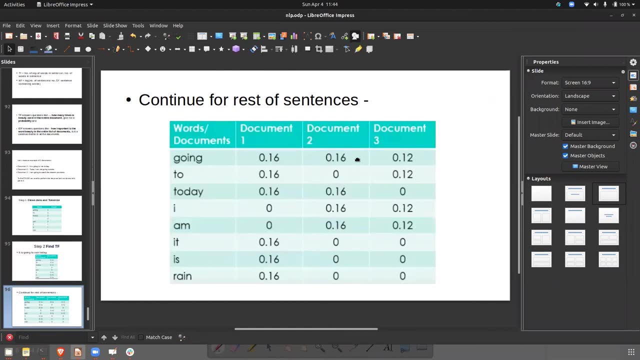 for each word is considering and it's calculating the tf for us. so this is the tf okay. remember, this is a tf okay. so this is a tf, this is so. this is a tf for national sentences. so when I say today I am it's rain, this is. 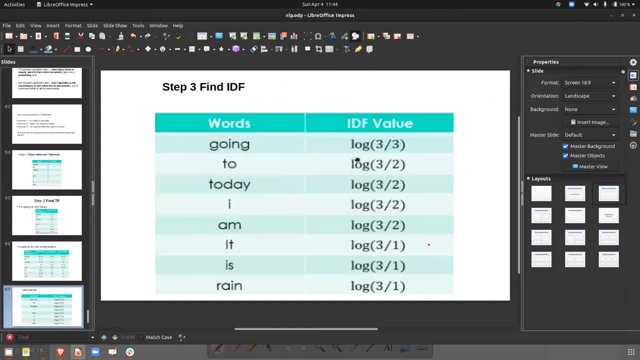 a tf for all the document. it's document 1, document to document three. this is IDR for each word. okay, so going to today, I am, it's rain, so this is the IDR for all the sentence or the vocabulary. For example, what does mean for know in teenage career what it means Monatee 14, Jas to 27 today.